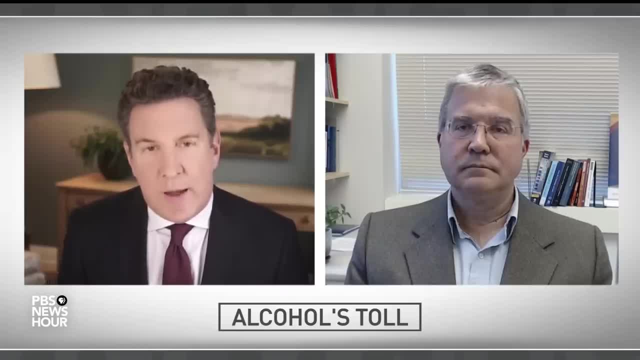 for Substance Use Research, DR TIM NAIMY, DR TIM NAIMY, Dr Naimy, great to have you on the NewsHour. Before we get to this changing guidance, can you just remind our audience: what do we know? 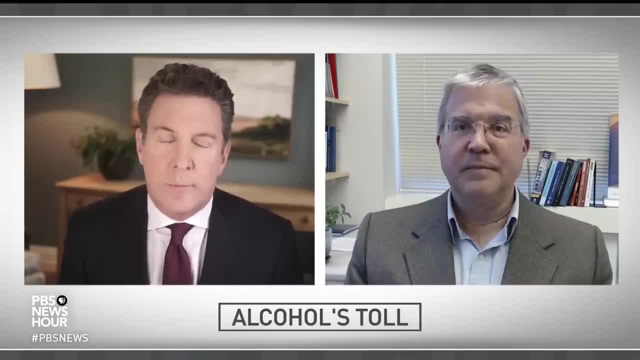 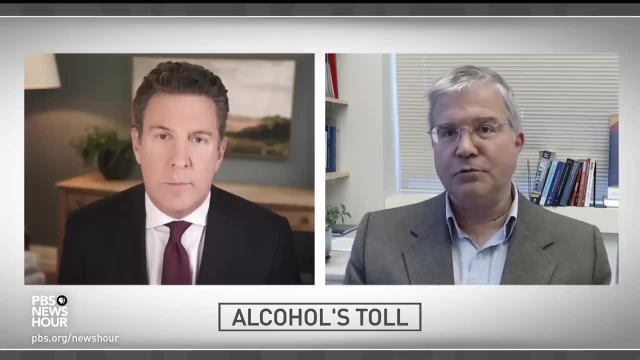 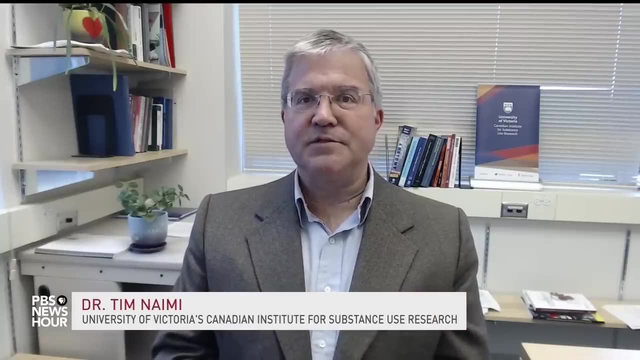 about alcohol's impact on us, DR TIM NAIMY. Sure, Well, you know, alcohol is one of the leading behavior-related causes of health problems and deaths and also some social problems and economic costs, you know, ranging from things like injuries and accidents to cancers and actually heart and cardiovascular disease. 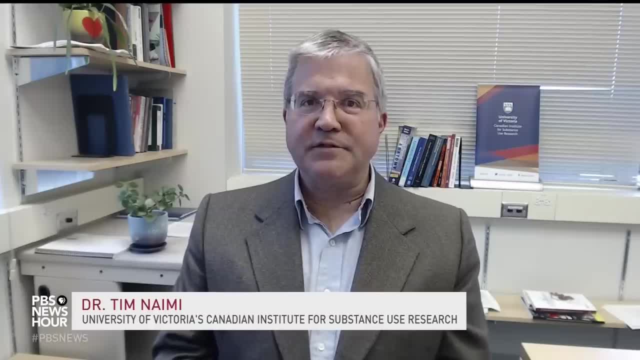 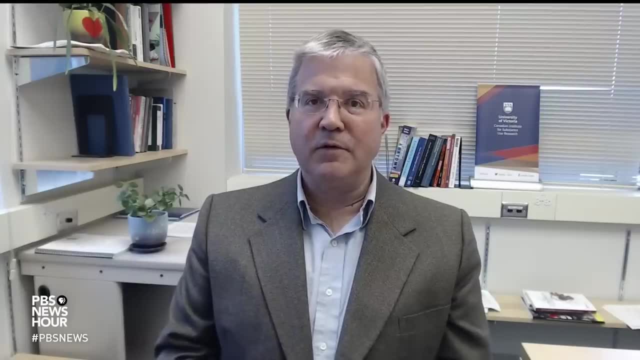 DR TIM NAIMY. So it causes a wide range of health effects, And of course those have been long appreciated at high levels of consumption, but even for some lower levels as well, And it also has impacts on our mental health as well, I take it. Yeah, well, there's a really complicated and important relationship between alcohol and things like depression and anxiety in particular. So, yes, so alcohol may play a causal role in those, but can certainly also, you know, exacerbate or make worse existing mental health conditions, particularly depression. 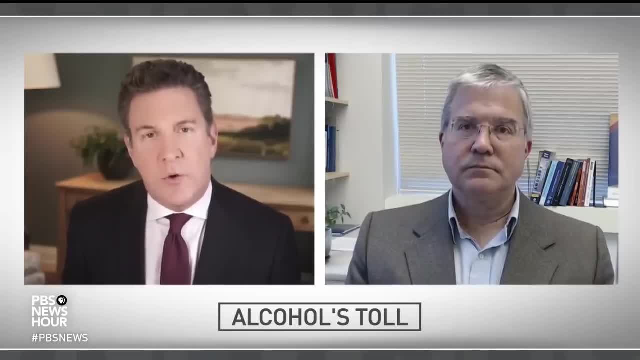 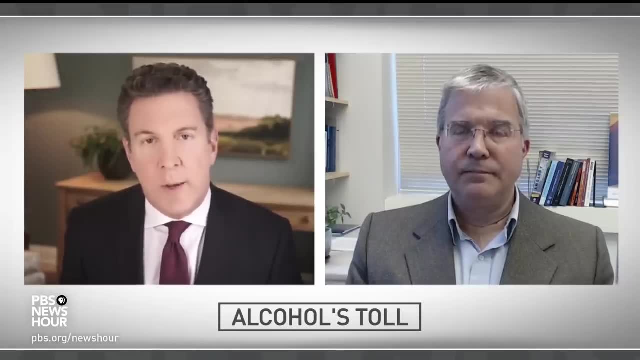 I want to talk about dosage for a second. You mentioned this in passing, but is it true that these harmful effects go up the more you drink? So a little bit is better than a moderate amount is better than a large amount. Exactly right, You know, when it comes to health, you know less is more. 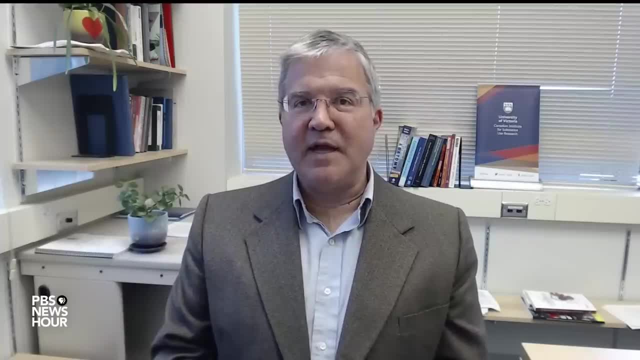 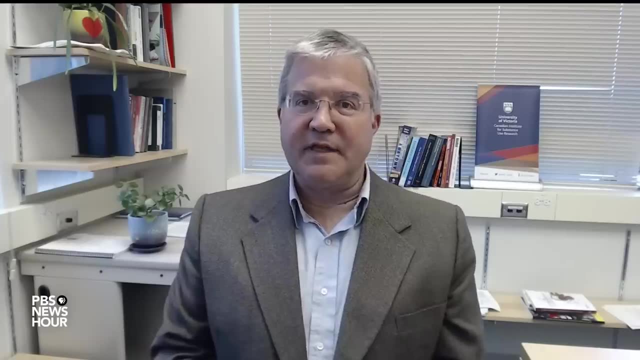 And that's actually the main thing, The main message stemming from the new Canadian guidelines. it's not that anyone needs to get down to a number. We know that the lowest level of risk is associated with a really small amount of alcohol. as little as two drinks per week is the lowest risk. 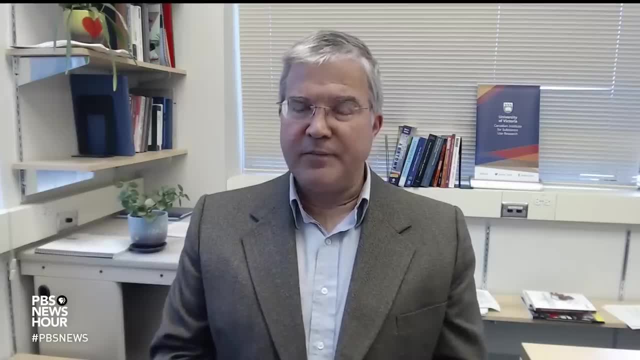 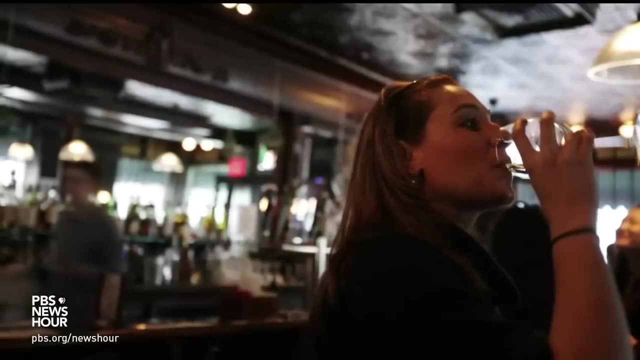 But the main message behind the new Canadian guidelines- and the main message- and this is, I think, is consistent with other guidelines- The big point to keep in mind is, no matter what level you drink at, that consuming less will be good for health, And we really want to reach out to people. 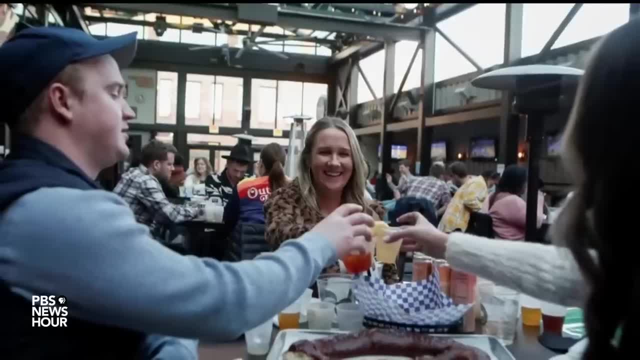 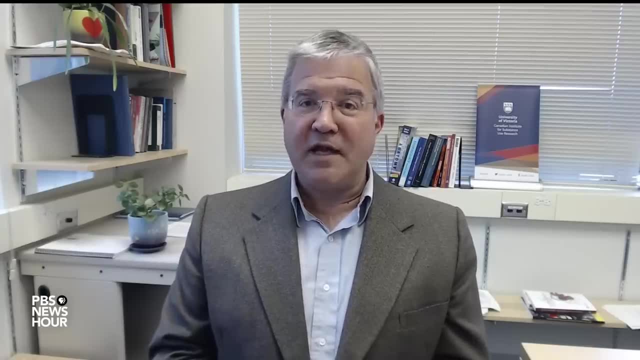 And I think this is we're talking about the public health community Broadly, not just to people who are already drinking a little bit and might cut back further, but people you know. if you're drinking six or seven drinks a day and you can cut down to three or four, that would be fantastic for your health. 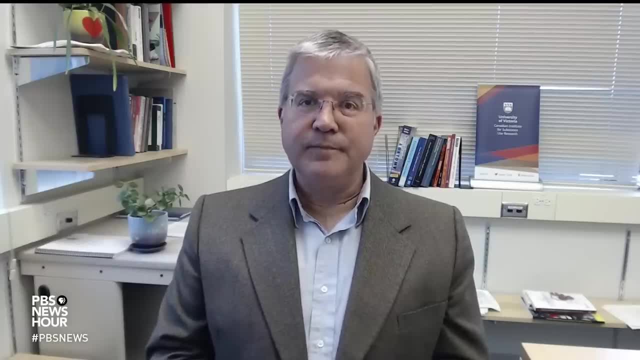 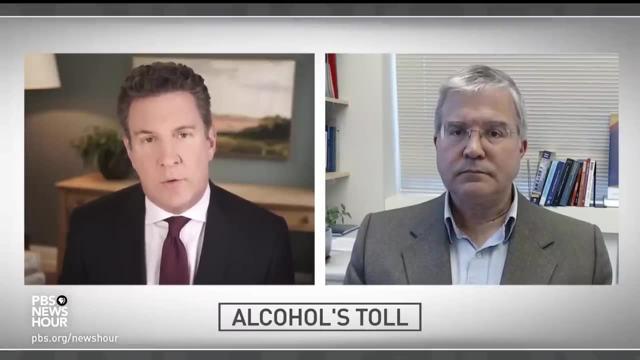 So just want to kind of reach a broad spectrum of drinkers. That's the basic idea. It still must come as a bit of a shock that something that is so widely accepted in our society can be implicated in cancer and heart disease and all of these other things. 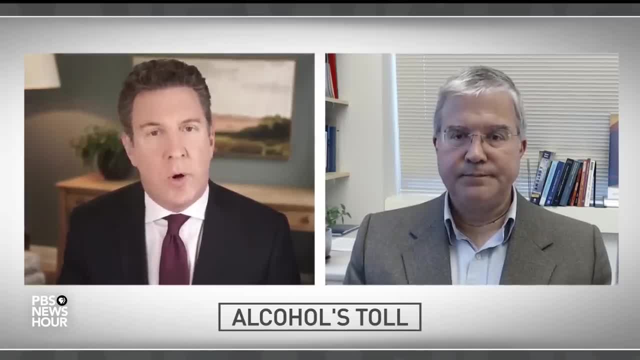 I mean, I think people think of drunk driving and they understand that It may be drunk and violence and things like that. But cancer and heart disease, do you think that the public fully appreciates those risks? Right, William? Well, I think you're right. 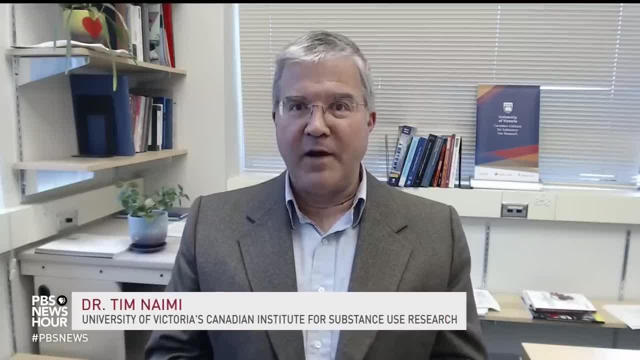 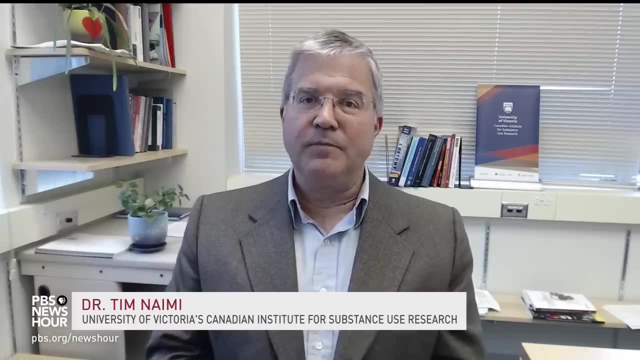 I think people are aware of. you know sort of impaired driving and crashes They're aware of. maybe you know cirrhosis of the liver And maybe they're aware of, like, fetal alcohol spectrum. you know birth defects and so forth. 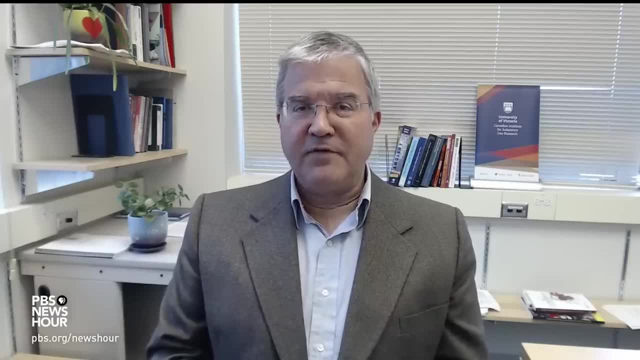 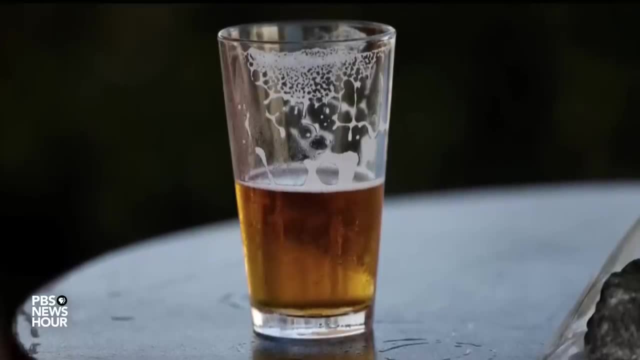 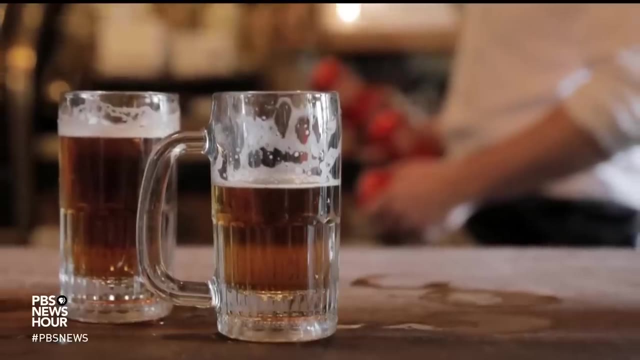 But I think they're much less aware of cardiovascular disease, And particularly in terms of the risk. I should mention that alcohol is actually considered a class one carcinogen or cancer-causing agent by the World Health Organization. So that's the same category as benzene and tobacco smoke. 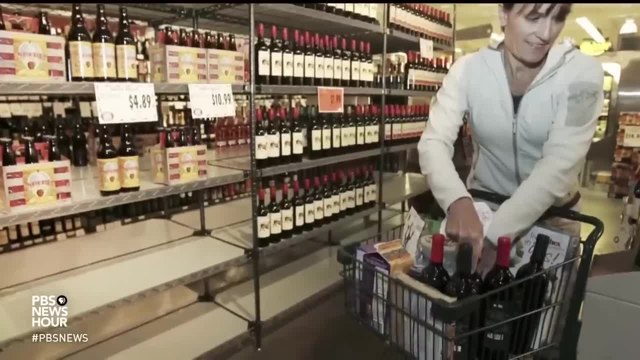 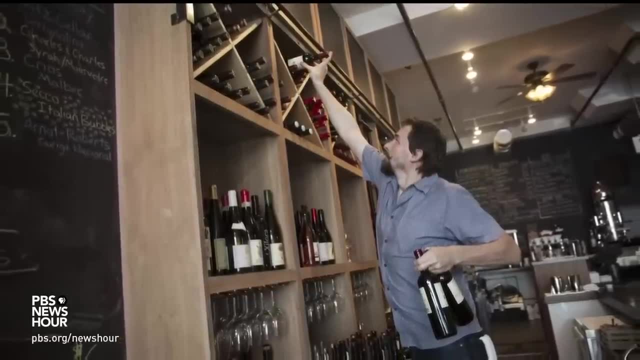 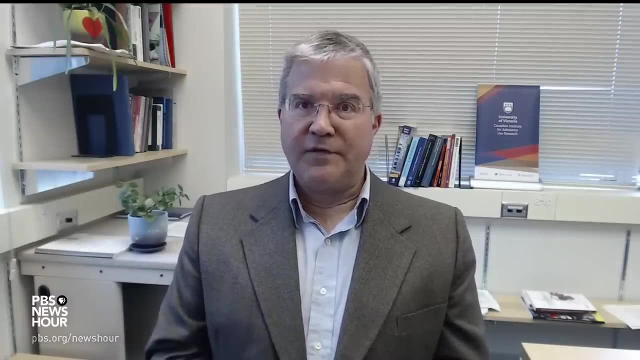 And some studies estimate that a drink of alcohol has about the same cancer-causing potential as one to two cigarettes, depending on your sex, You know. as an example, the risk of breast cancer goes somewhere between 8% and 10%, increased with each additional drink. 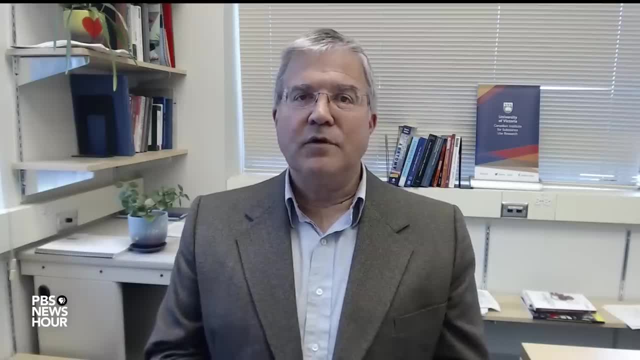 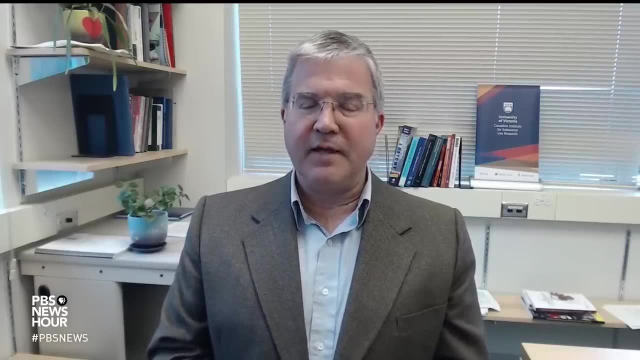 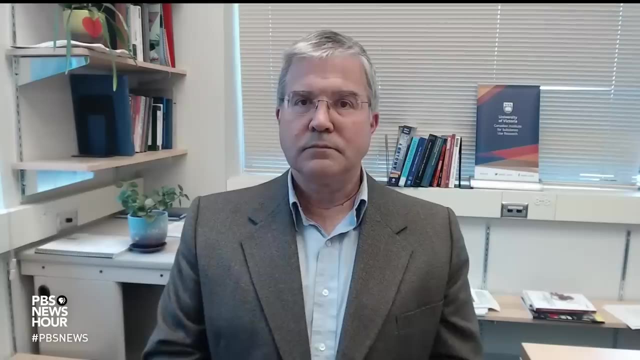 So that's an important thing, And we know from surveys that only a small fraction of the population understands the cancer link. Help me understand, though. It feels like we've been getting some conflicting guidance. I think many people remember being told that moderate amounts of drinking for certain people can be beneficial. 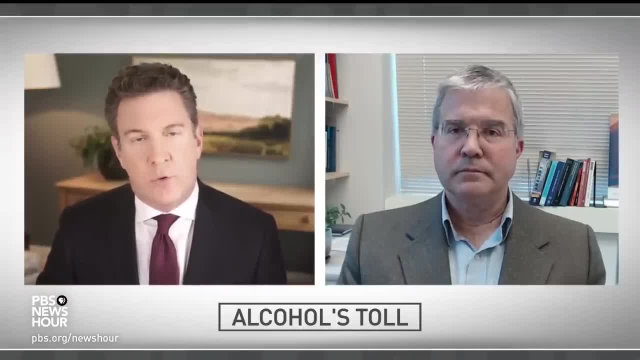 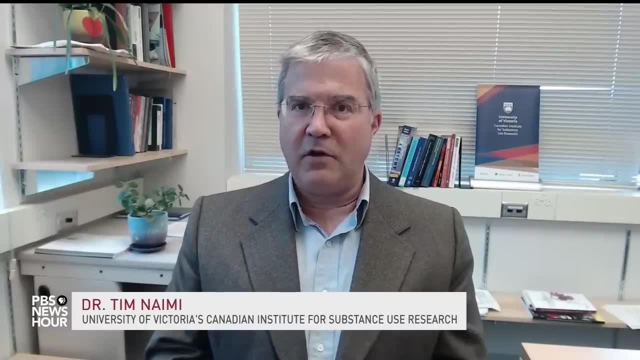 There was that infamous study years ago that red wine was good for your heart. Are those things? just have those gone by the wayside now? Even for those studies, above very small amounts of alcohol, the risk started to increase. So it's really an argument about how low is that point? 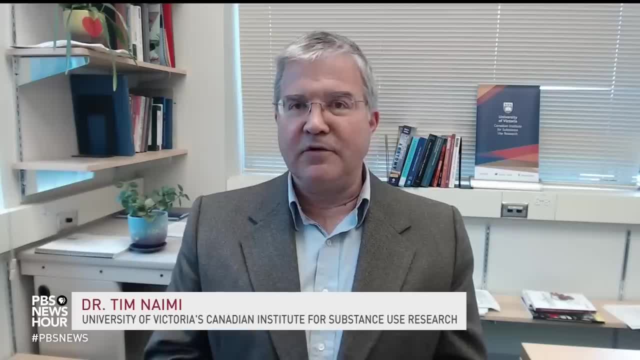 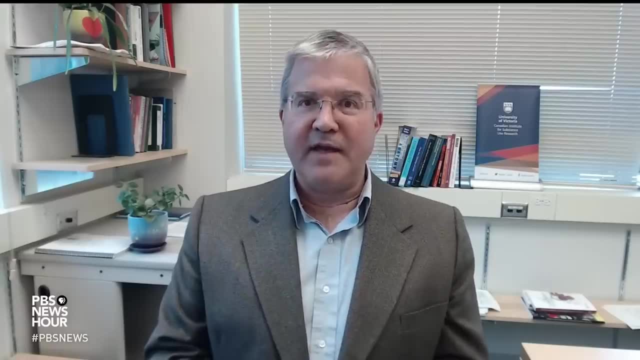 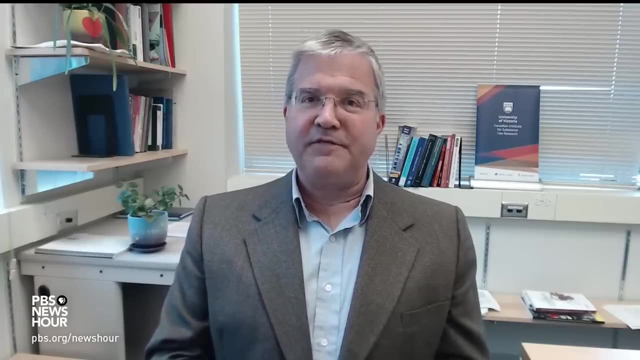 So, broadly speaking, I think the science is consistent that that sort of less is better, down to very low amounts. Yeah, I do think. I do think some of that science has gone by the wayside and without getting deep into the weeds, The basic idea there is that that somebody, for example, a red wine drinker in their 50s who's been drinking just a small amount for their whole life, 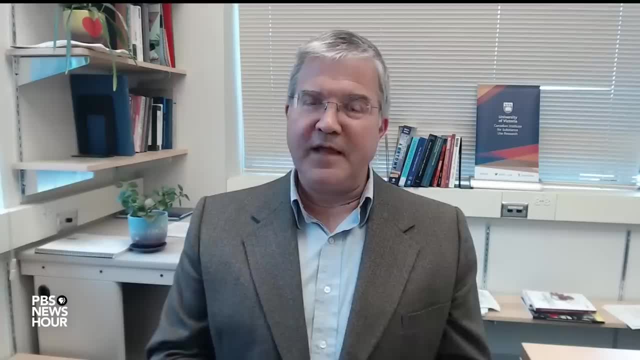 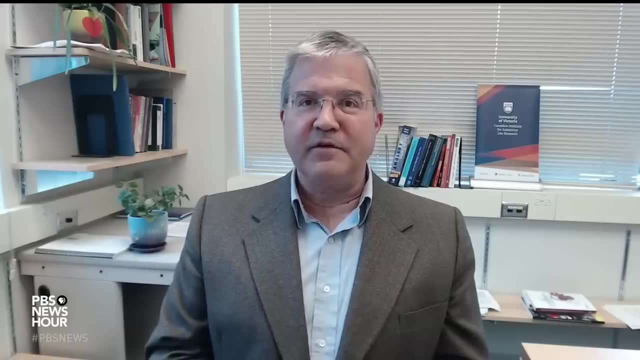 is actually somebody. those people tend to be super healthy and have a lot of social advantages And and so maybe their red wine is a reflection of that and but not its cause, And that's the basic problem with the previous research on that. As I mentioned, a lot of Americans are doing this dry January.